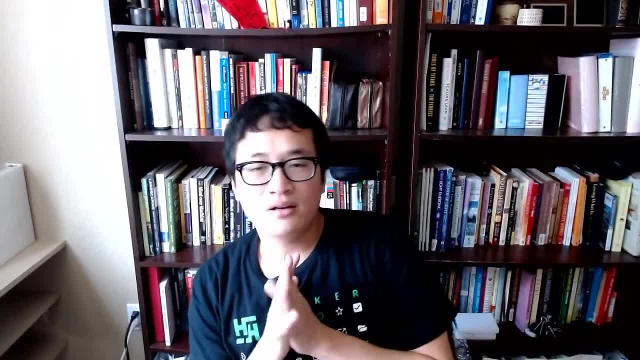 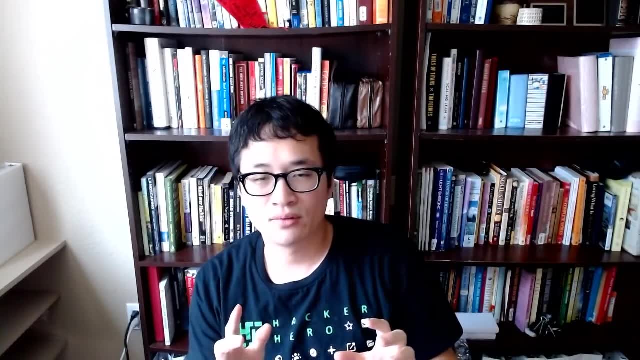 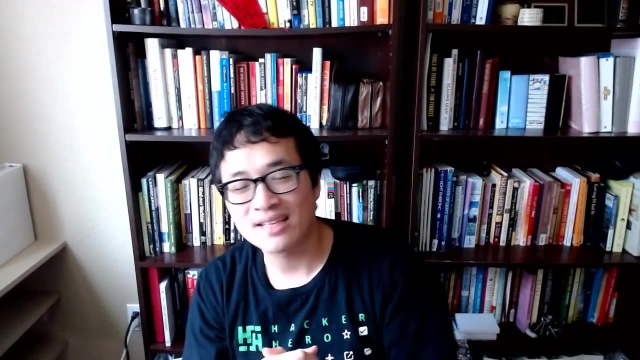 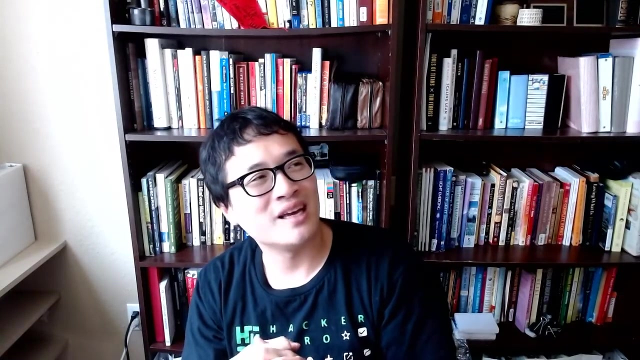 All right, so let's talk about the core building blocks of programming. Every software that you've used is really built with what I would say five core building blocks. That's it. Everything in the world that software is created using those, And I think of it almost as Legos. These are the 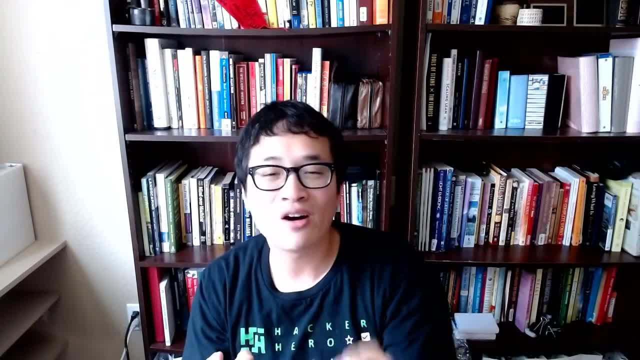 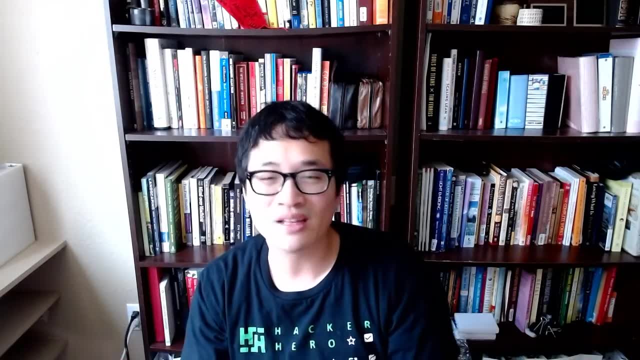 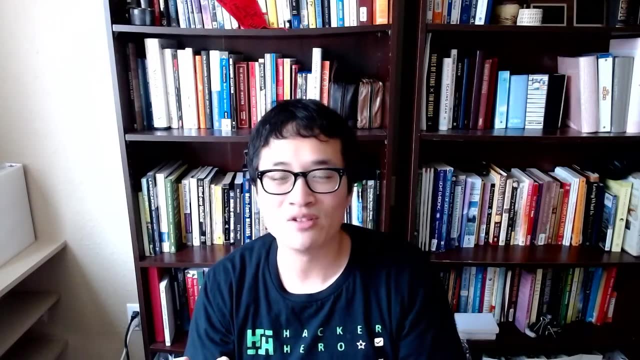 fundamental Lego building blocks to create anything, whether that be a car, airplane or, in the software space, a site like Amazon, Facebook, Google, any of the websites that you've used, any of the mobile applications that you've used, any platform that you've used on PlayStation. 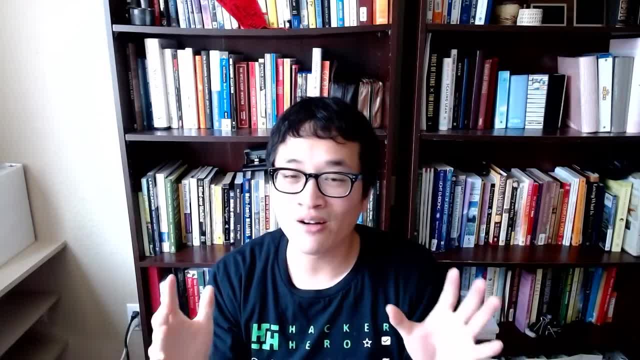 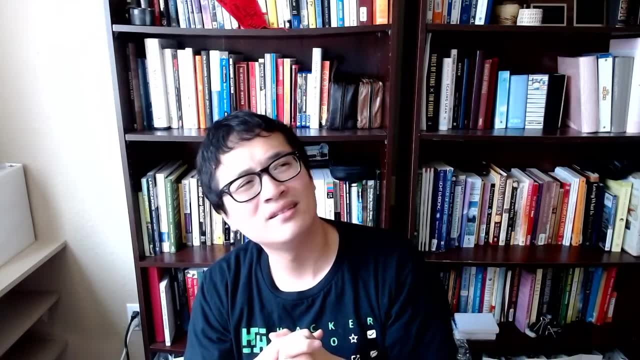 Xbox, whatever anything, software games- they're all built using these five building blocks. That's it. It's almost like there's a movie about the Legos, right? I can't remember on top of my head, but there is this master builder, I think. 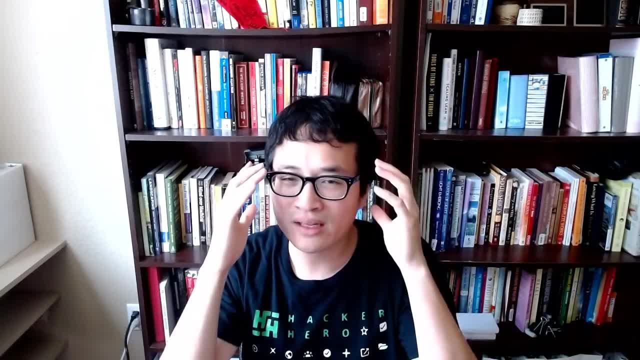 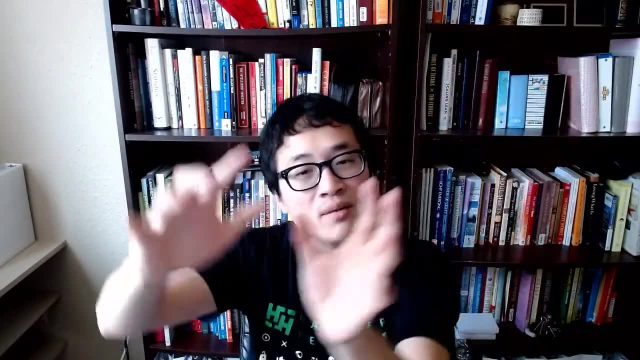 and they can build anything they can think of. A good programmer is able to look at a problem and say, oh, if I just put these five building blocks this way, I can create this. And then if I build it this way, I can create this. That's how it works. So what are those core building? 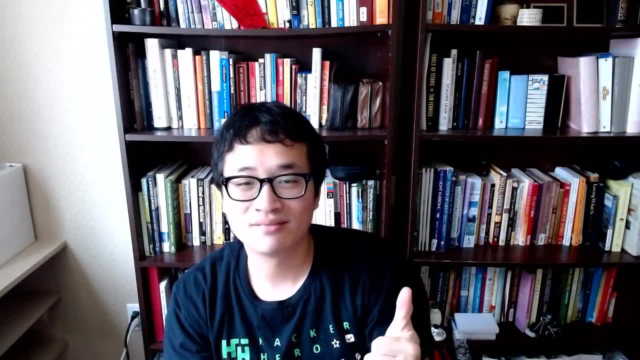 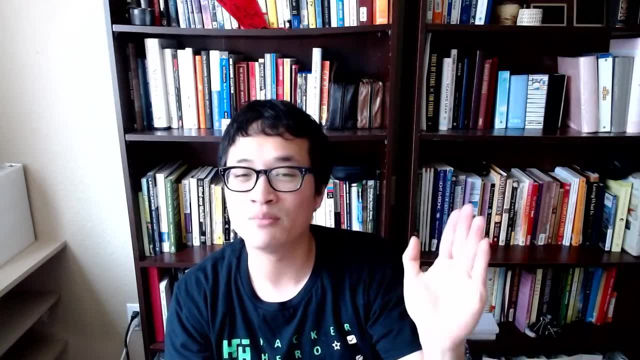 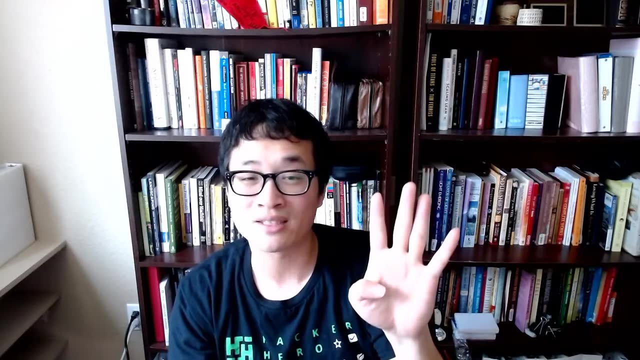 blocks, If and else, statements, loops, functions, understanding variables- especially how arrays work, and then object-oriented programming. This class is going to cover the first four And the algorithm app is going to help you master the first four concepts And then later object-oriented programming, or OOP as what people call. 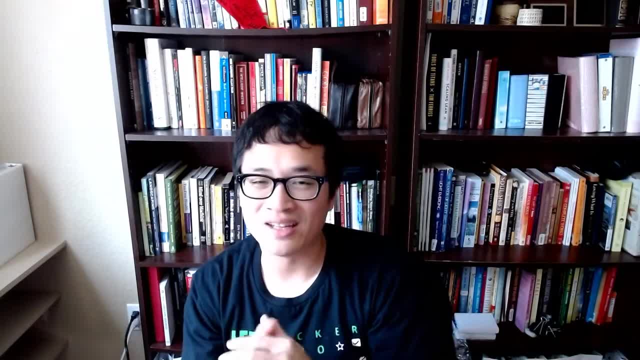 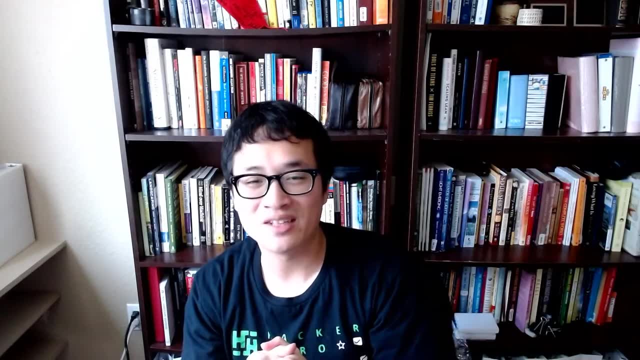 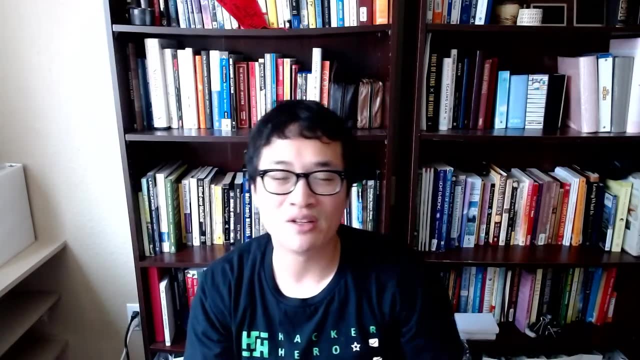 will be easy for you to learn, And that's another breakthrough I had. After years of iterations, I finally figured out how to teach OOP in about seven minutes, So I'm really proud of that accomplishment. So I'll share that video later on, But anyway. 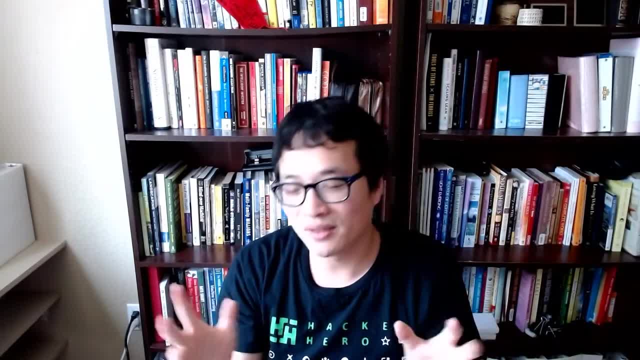 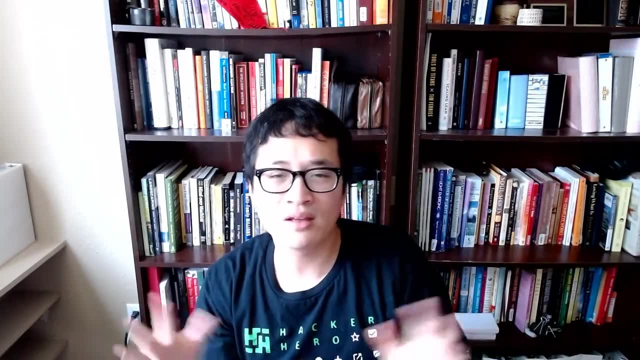 everything in the world is really created. Now, you may find that hard to believe. I probably found that hard to believe if I was learning to code for the first time and someone told me everything in the world is created using that. But I'll prove it to you And later in the